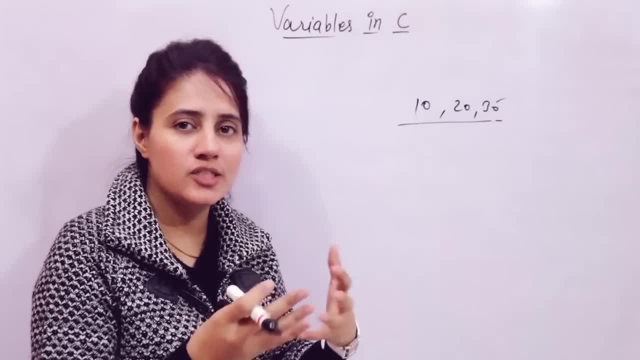 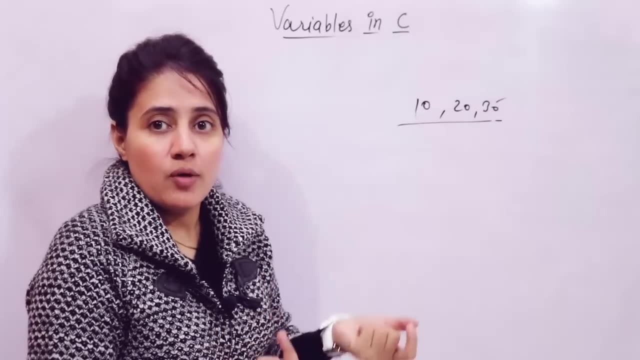 program right In programming language. you need some programming language. You will write program and you will submit that program to computer And then you will get output like maximum number is 30. So now computer is not not having its own brain, its own like memory. Yeah, it's having its memory. 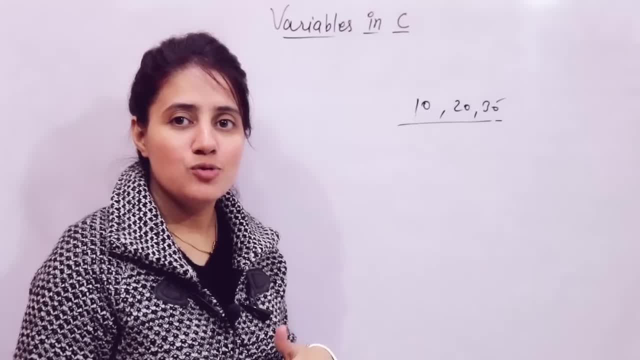 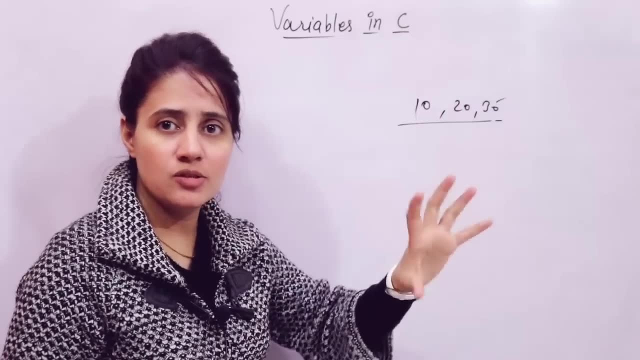 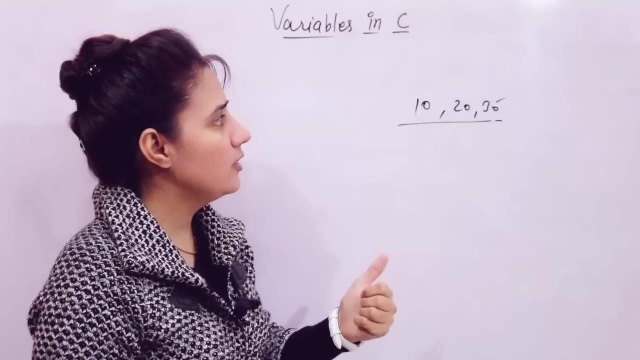 But it's not having its own brain like we human have. So there, you need to store these numbers in computer memory. Obviously, computer need to store these numbers in his or its memory. So now, to store these numbers, or to store some values, what you need, you need a variable name, like C, Suppose this is memory like 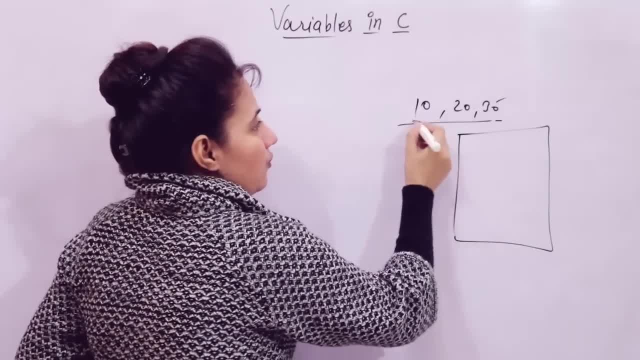 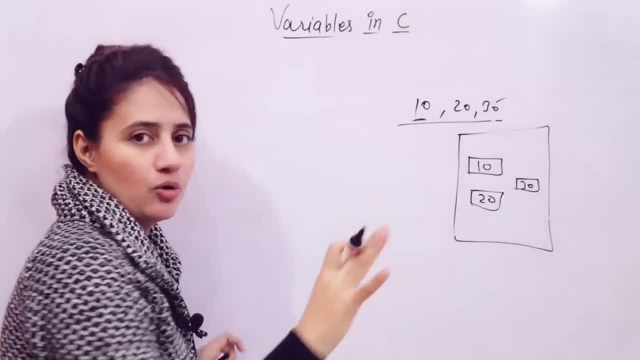 computer is having a chunk of memory And if I want to store 10, suppose I have stored 10 here, 20 here, 30 here, Any random locations in computer memory, these numbers will be stored in any random locations, right? These are having some addresses, suppose addresses, suppose addresses thousand, this address, right? 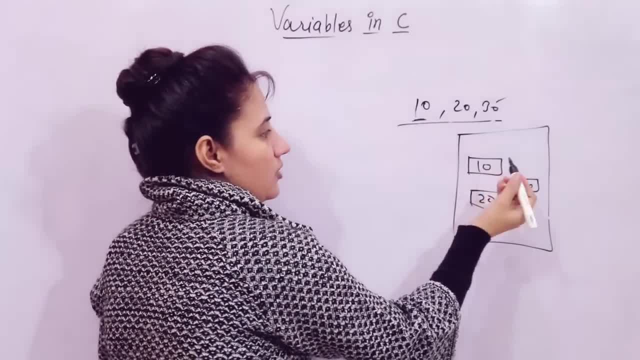 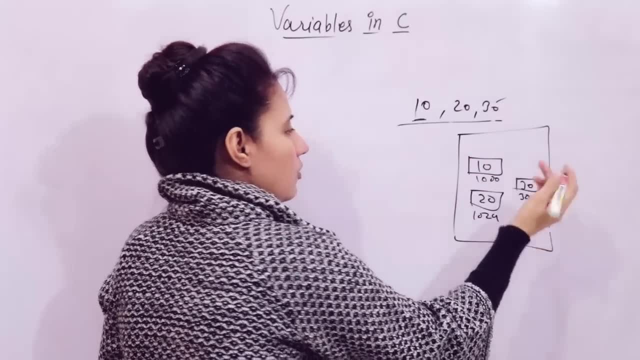 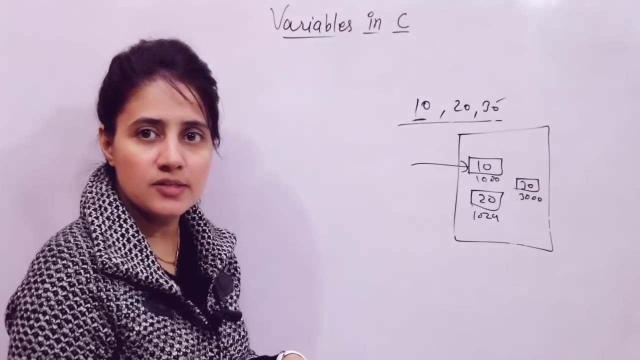 These are having some addresses, suppose addresses, suppose addresses thousand. this address right. This address right is suppose 1024, this is 3000, any address right now. if you want to access these values, how you will access, because you are having. we don't know where these numbers have been stored. 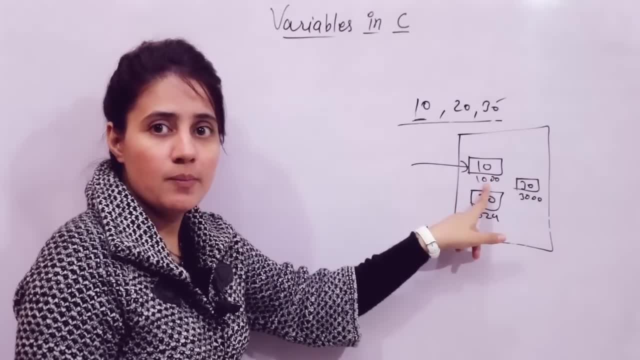 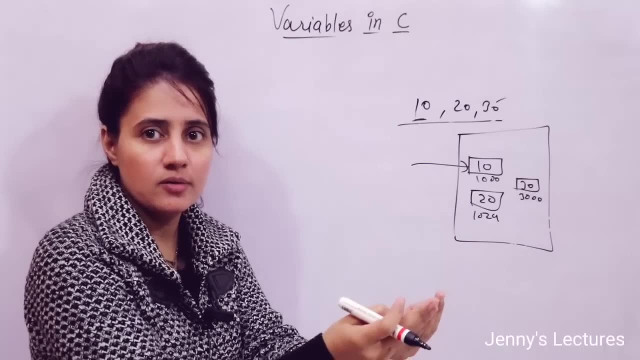 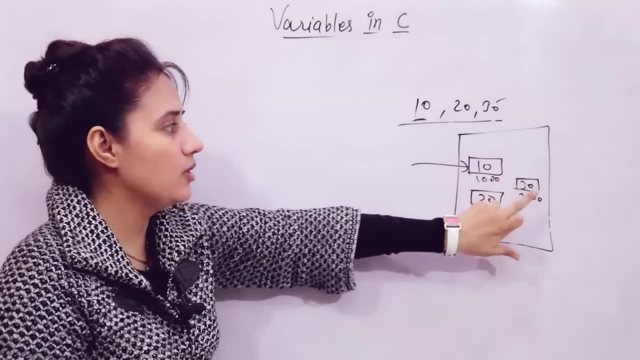 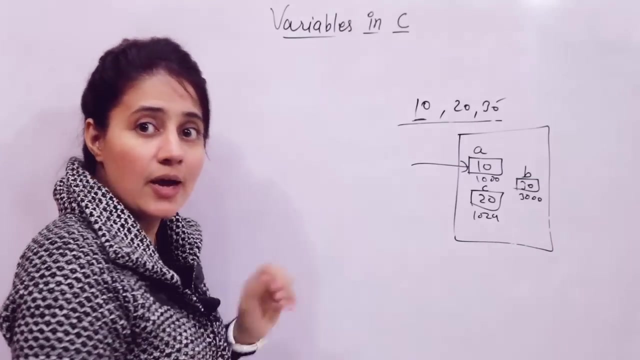 either you have to check for these addresses, but generally we cannot open that memory, we cannot generally touch the memory locations in computer right. it is not possible. so what we can do, we can give a name to all these three memory locations, like suppose I am giving name A to this, B to this and C to this. now if you want to access these numbers you can. 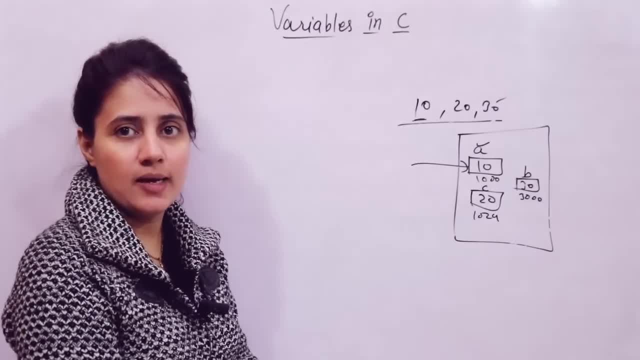 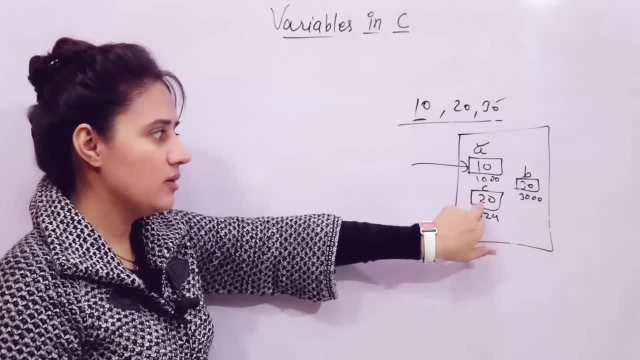 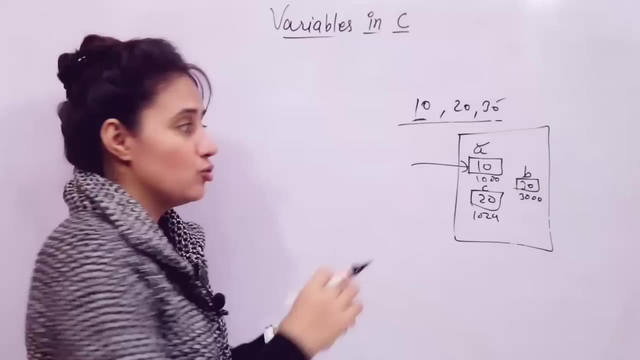 easily access by calling the name only like A fine B. when you call B, then 30 would be displayed. and when we print C, call means when we print C, then 20 would be displayed. we can easily call it like that. So these A, B, C, these are what variable names, these are variables. so variable is what it. 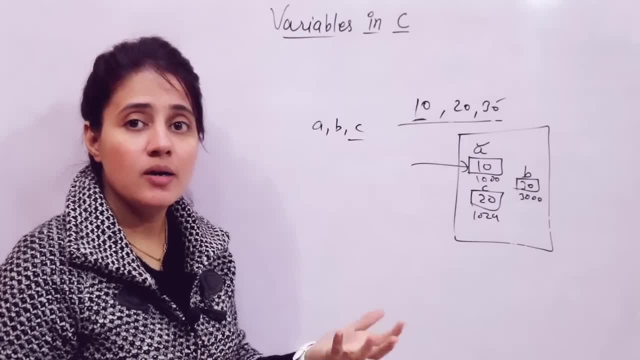 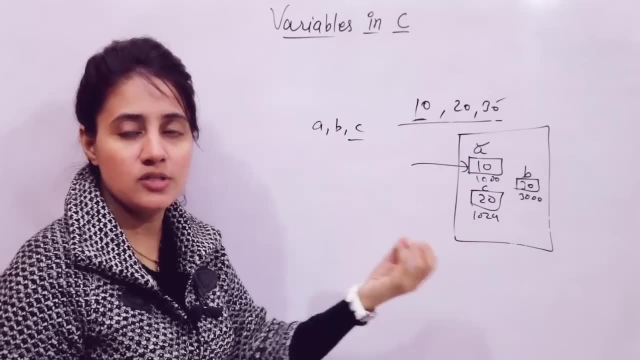 you can say a named memory location. it's nothing but a named memory location. this is a memory location and it is having a name A. this is variable A, it is a named memory location. or you can say: a variable is what? it's a name or it's a data name that is used to store. 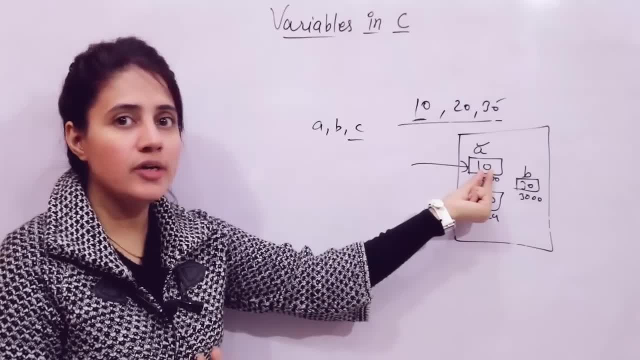 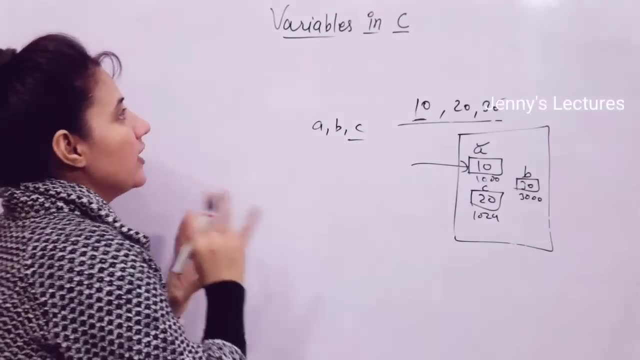 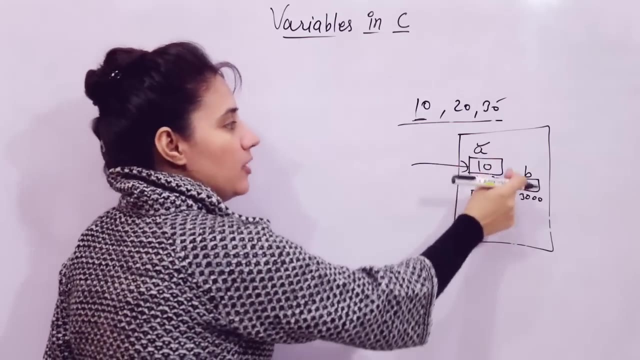 what value of data. Here I am storing value 10, right, and the name is A. this is variable. fine, now let us discuss how to declare variables and see you can also say: variable is what it's: a name which is given to a memory location where we store a value or any constant. this is what constant. 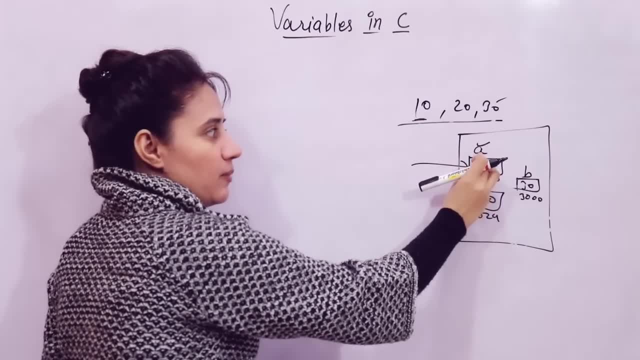 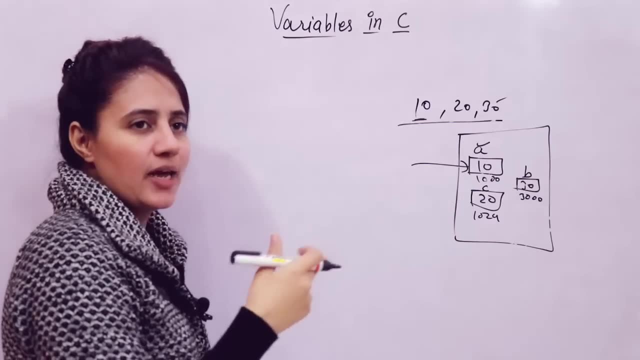 right. so I am naming this memory location that is A, and I am storing here value of a constant, fine, So name of a constant, So name of a constant, So name of a variable. generally we declare anything like A, B, C or anything but suppose. 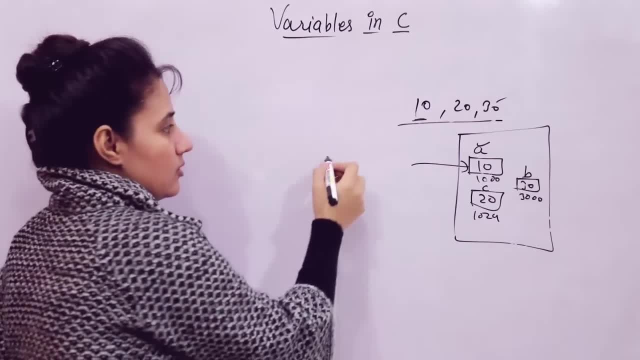 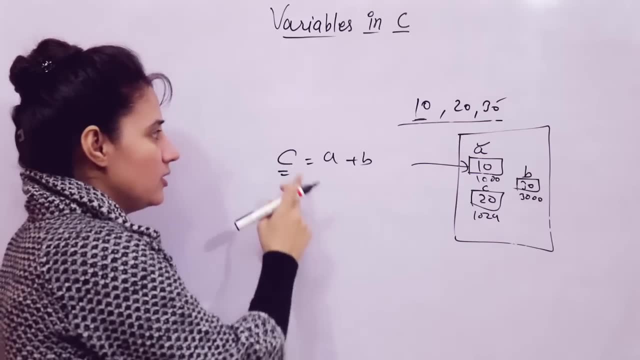 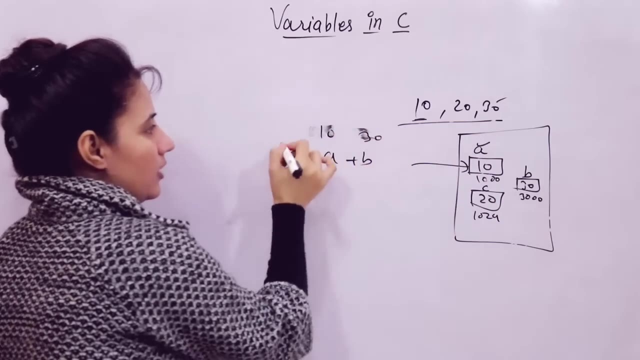 I want to print sum of two numbers, A plus B. So rather than writing C here- yeah, you can use C here and you can print C- then sum would be printed like: A is 1, suppose, and B is 2, or here I can say: A is 10 and B is 30, then in C we will have 40, but rather than 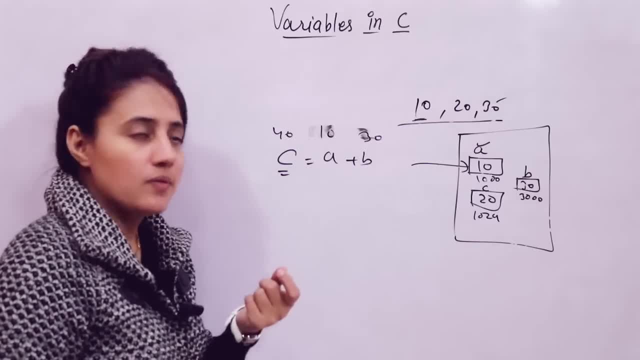 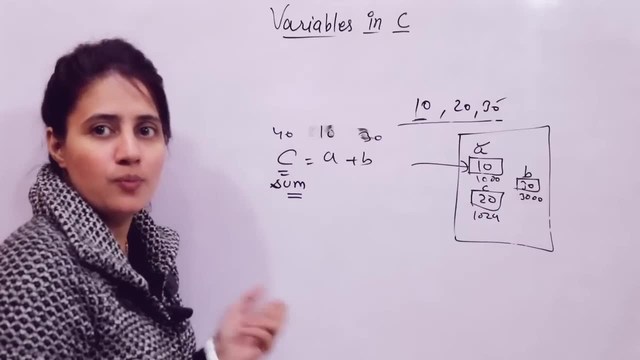 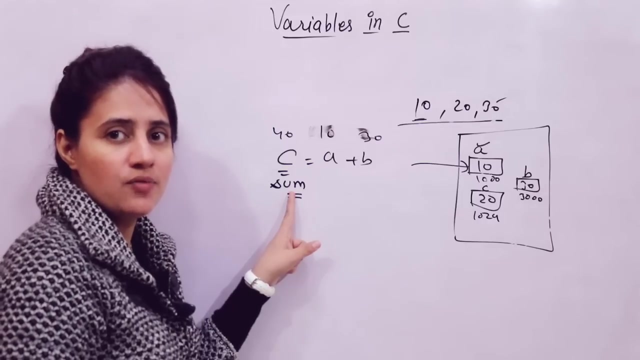 writing C programmers you do what They write down a meaningful name. like if I write down here sum, that would be more meaningful. just by seeing the name, the name of this variable, you can easily find out, you can easily figure out that this is what this variable is containing. sum of numbers may be two numbers or three. 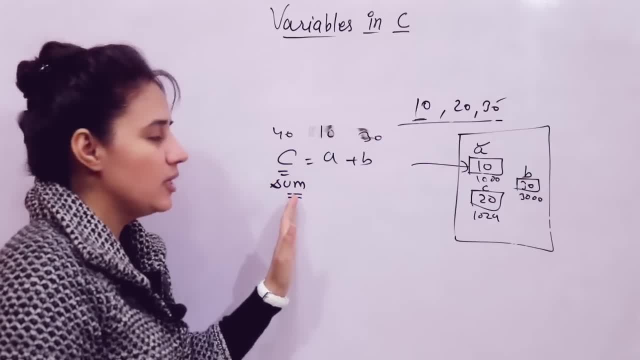 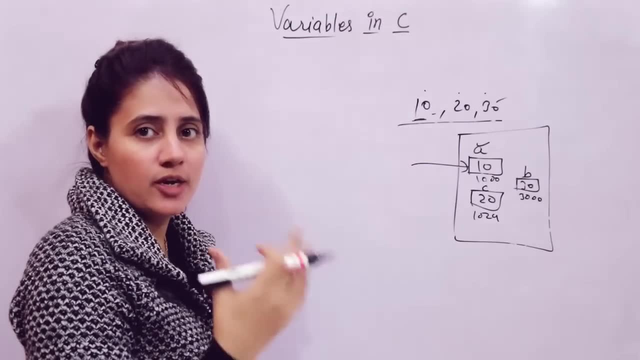 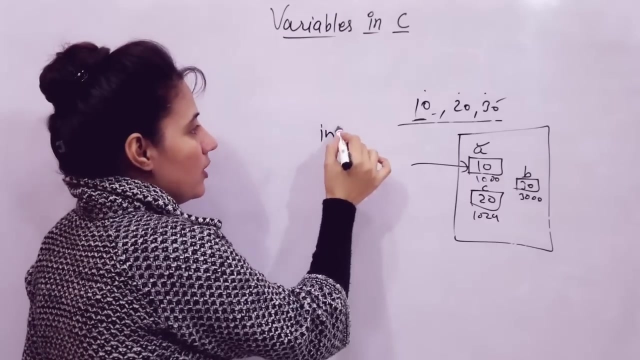 numbers. here it is containing sum of two numbers, So better to use a meaningful variable name and, as the name suggests, variable means the variable, So the value of that variable may be changed during the execution of a program, means throughout the program. In the previous video I have discussed also like: if suppose I am taking, A is equal to 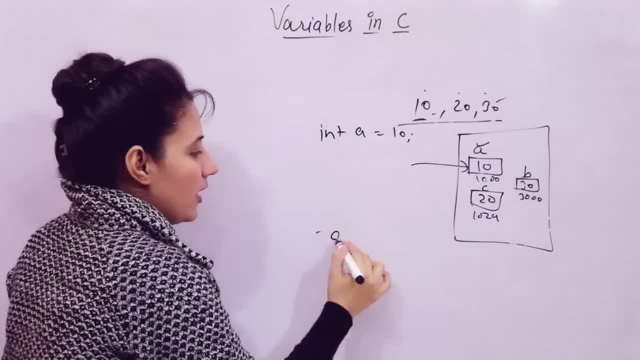 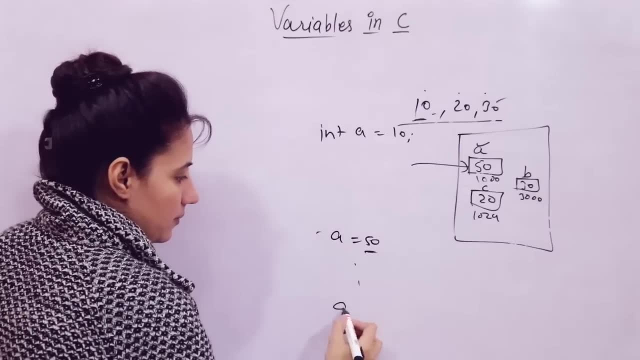 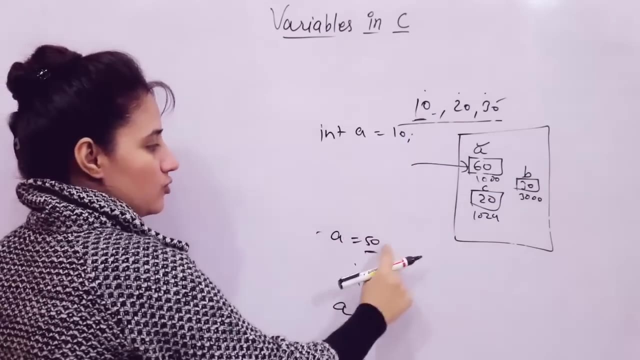 10 here. so in this program, anywhere I can change, A is equal to 50 and that value would be updated to 50. now, If, after I am writing, A is equal to 60, after that A value becomes 60. this value has gone. this value has gone. 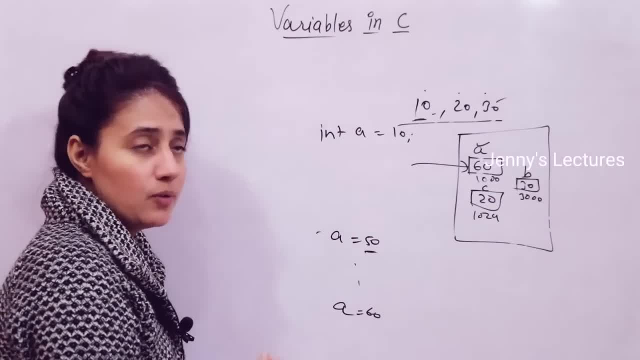 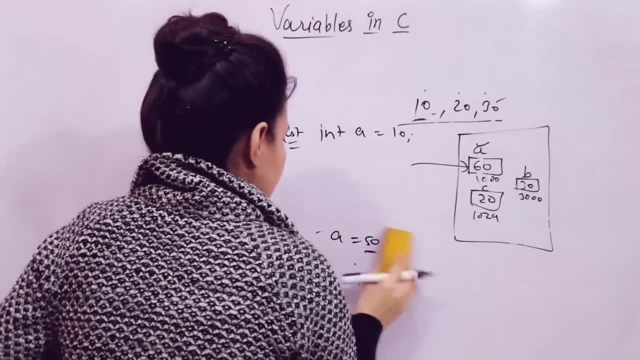 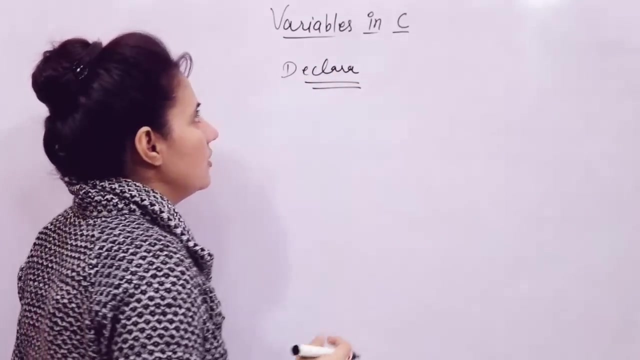 Now updated value is 60, so you can change that variable value. but if you define like here, const now, you cannot change the value. it is like a constant variable. fine, that I have discussed in previous video. Now let us discuss how to declare a variable. we will also see declaration and initialization. 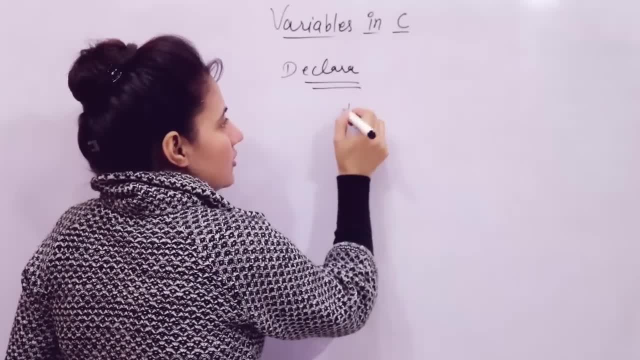 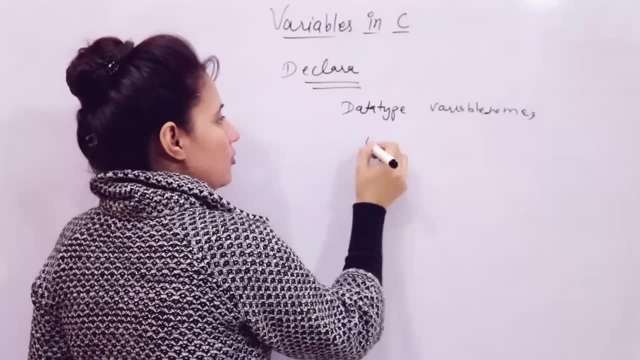 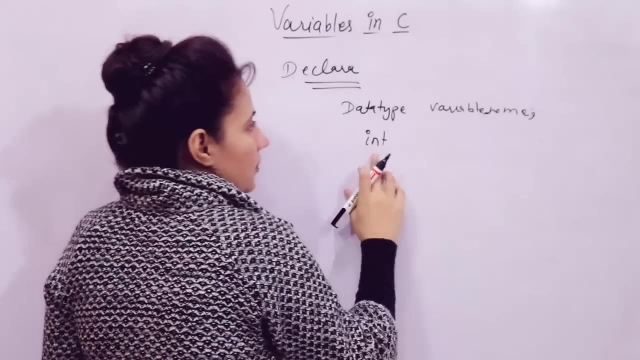 See for declaration we need what? two things: first is data type, second one is name of that variable. So here I can write: suppose data type is int data type, you can write int float character- that data types also we will discuss in the next video- and variable name. suppose I am writing. 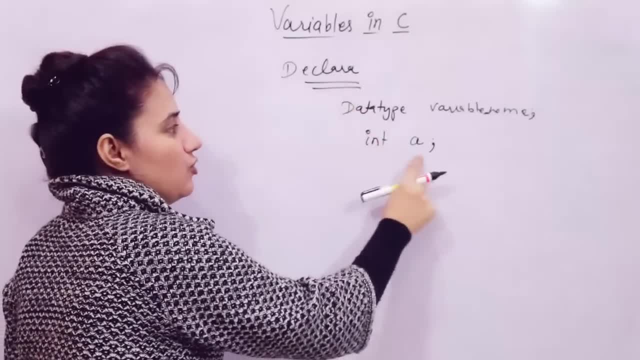 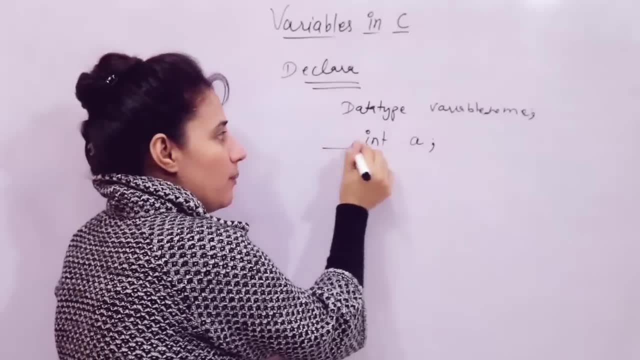 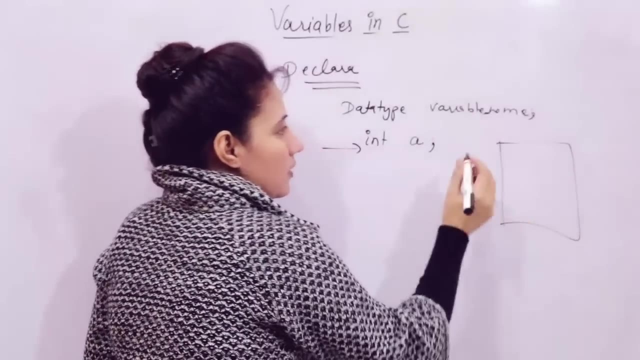 A and then semicolon. this is what declaration of a variable. So it is telling. the name of that memory location is what he. if you write this thing and when compiler will compile this thing, when compiler, the control, will come to this point during execution of a program, then what will happen? It means: 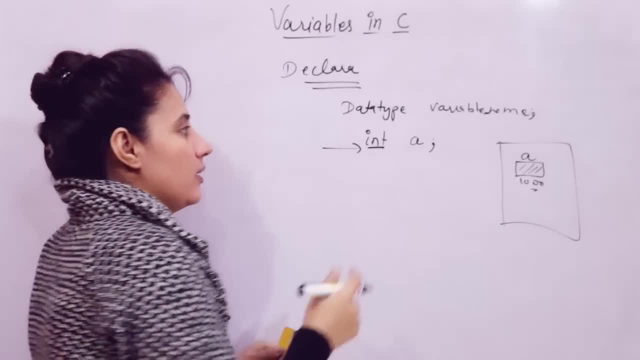 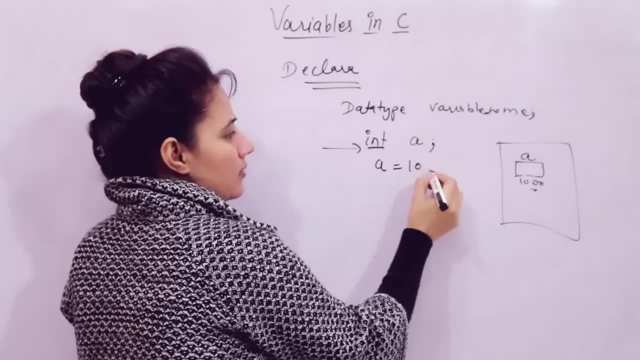 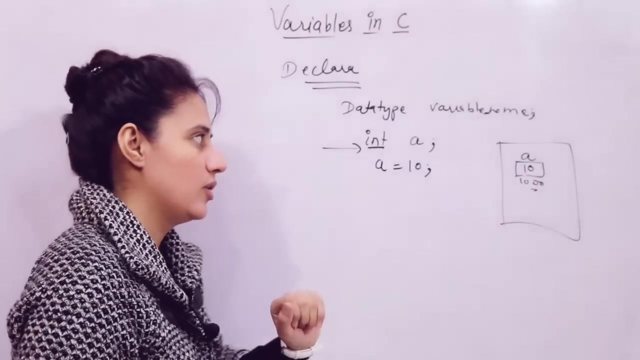 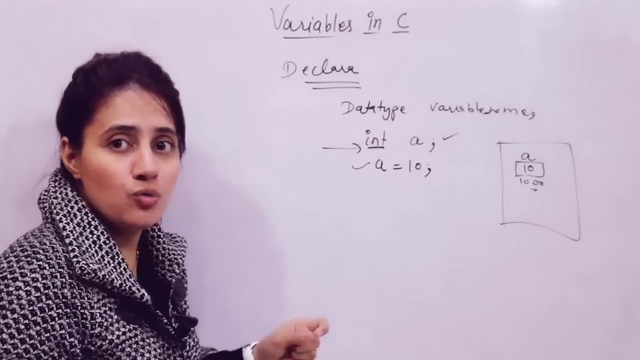 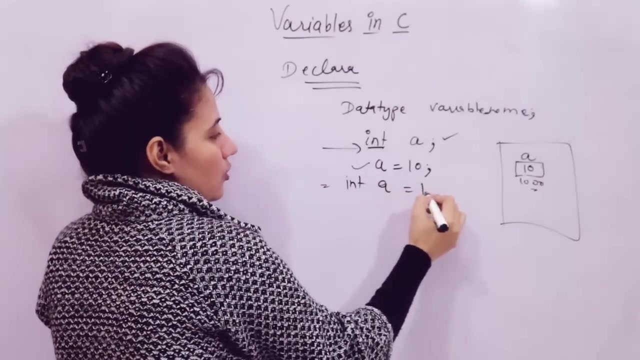 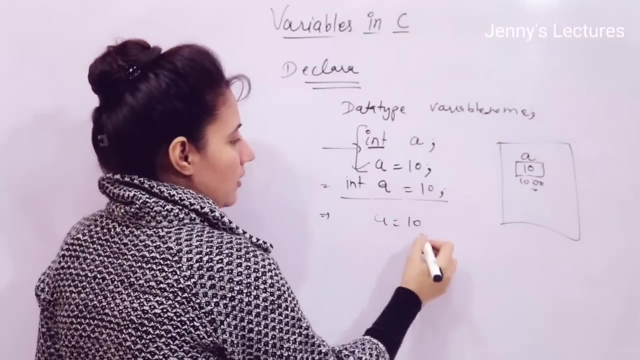 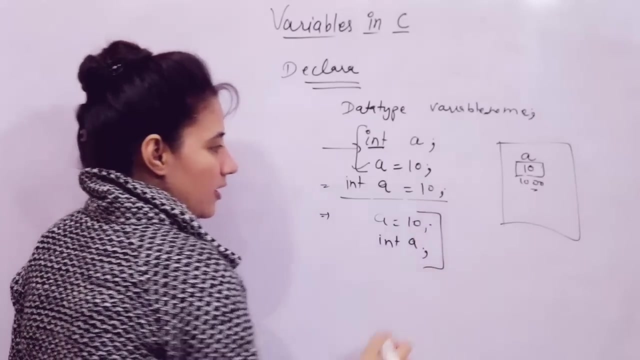 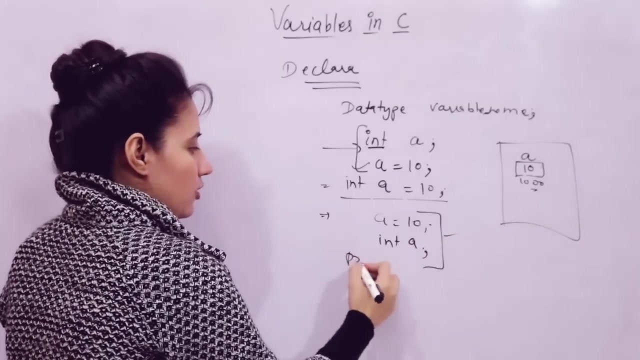 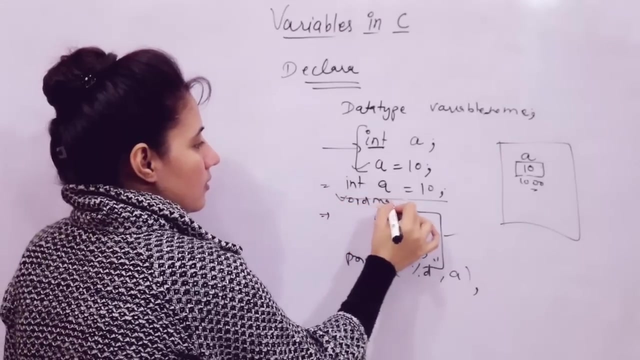 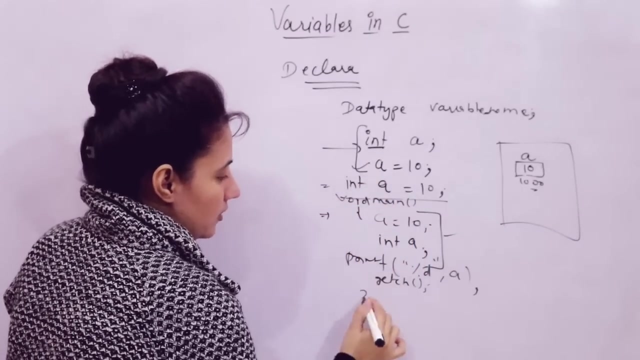 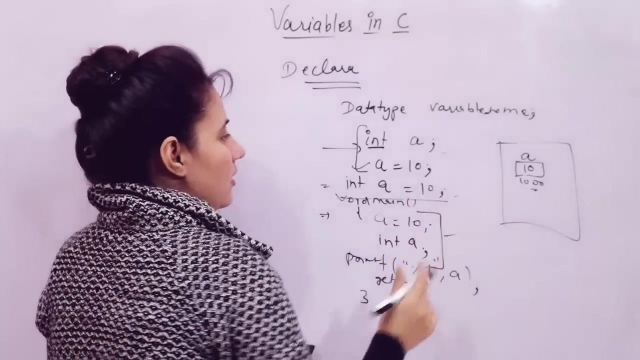 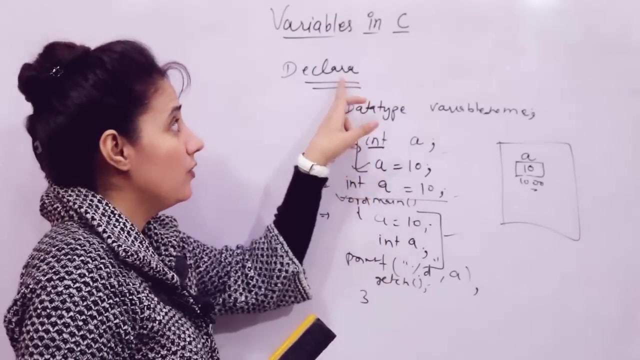 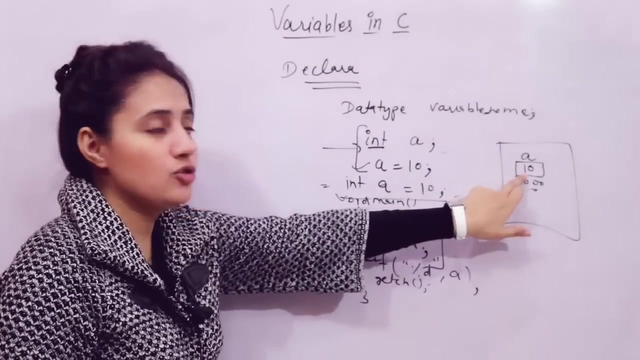 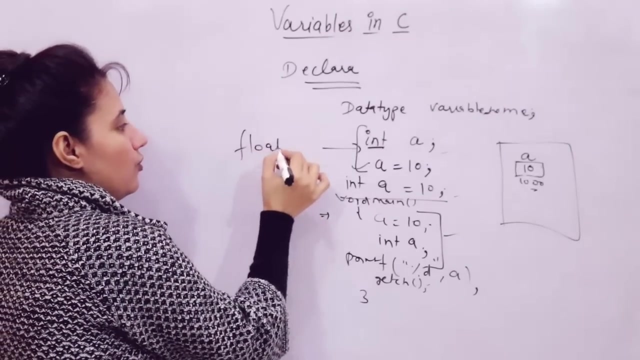 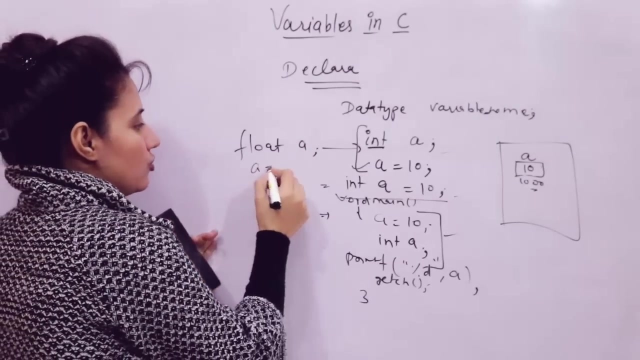 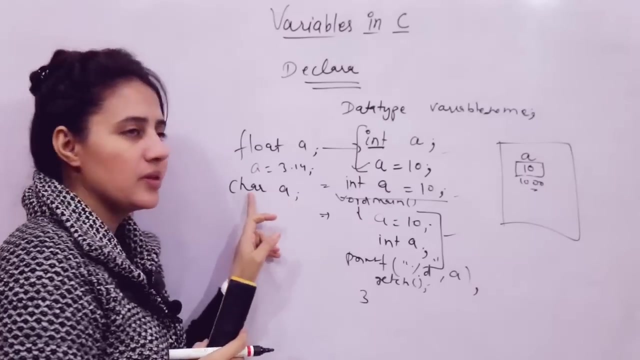 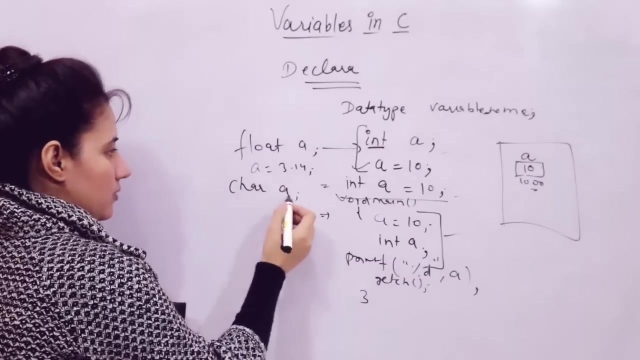 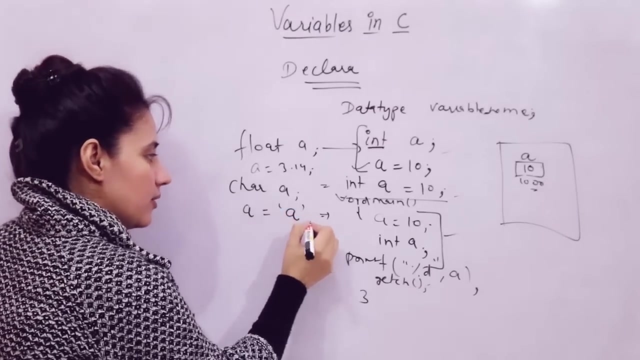 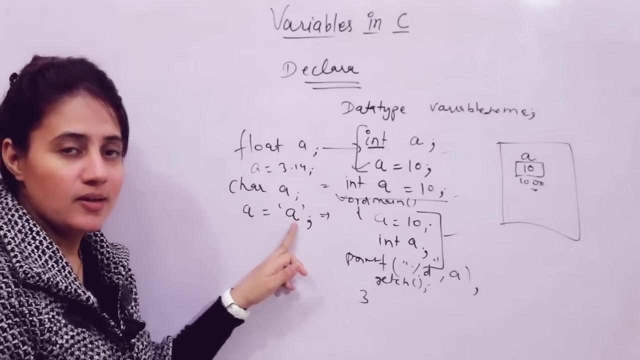 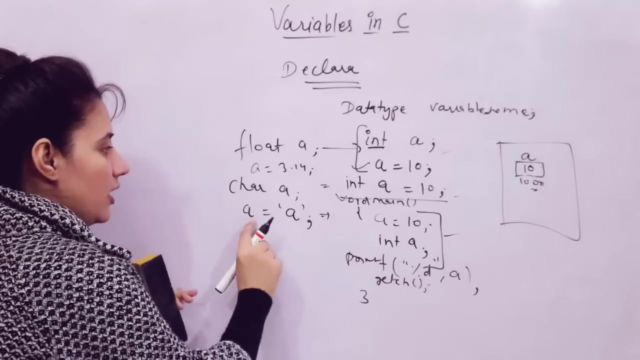 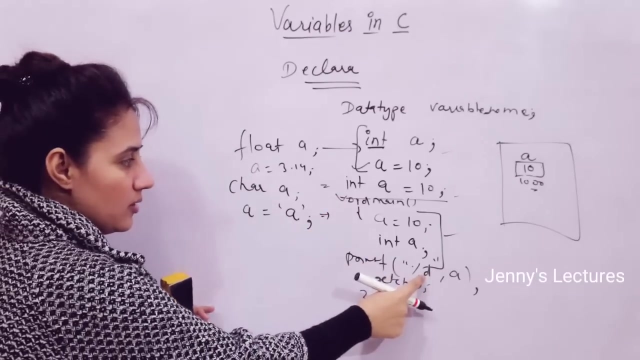 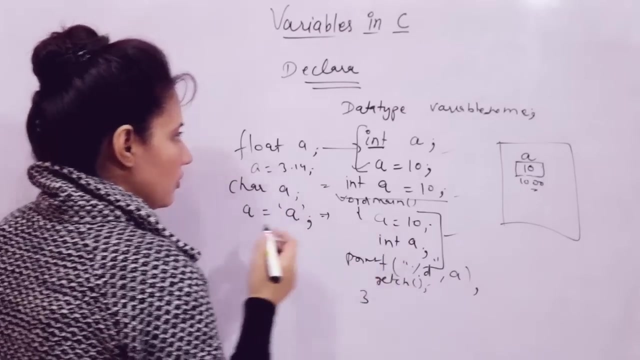 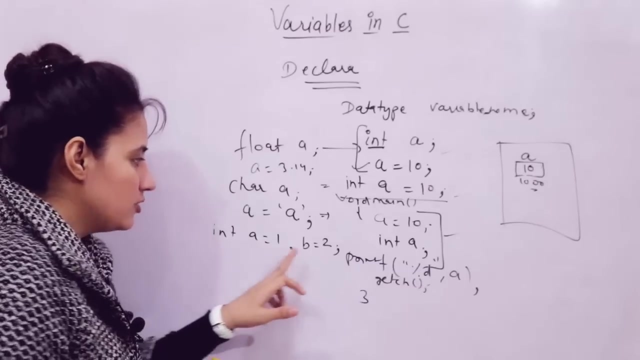 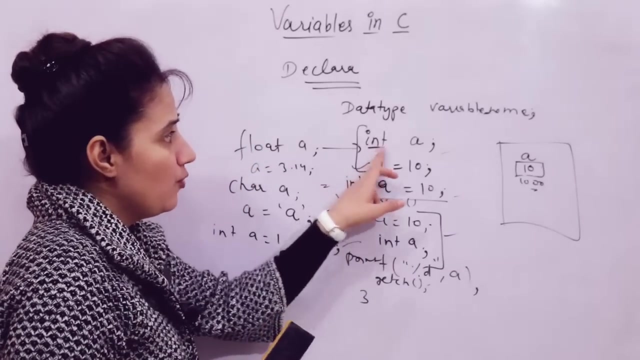 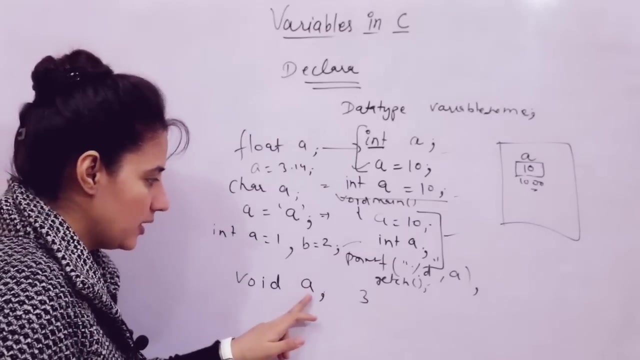 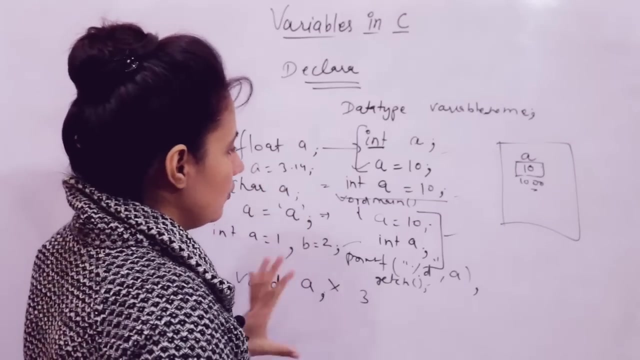 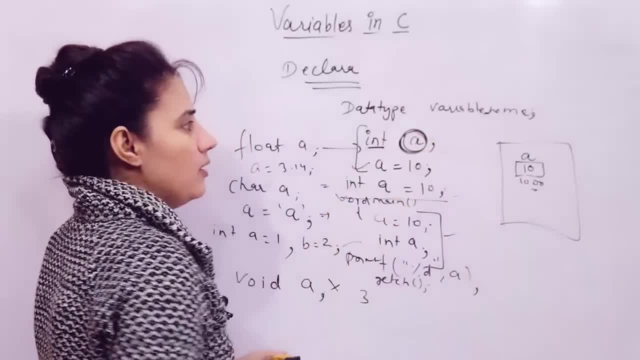 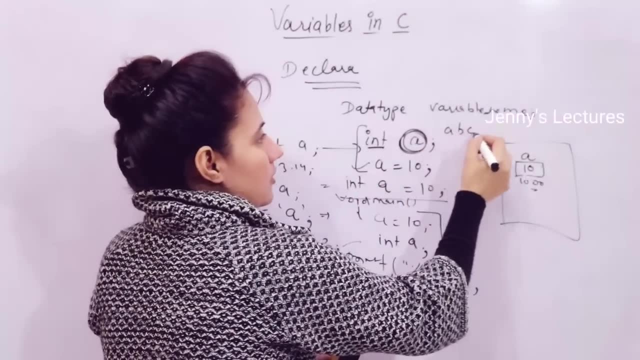 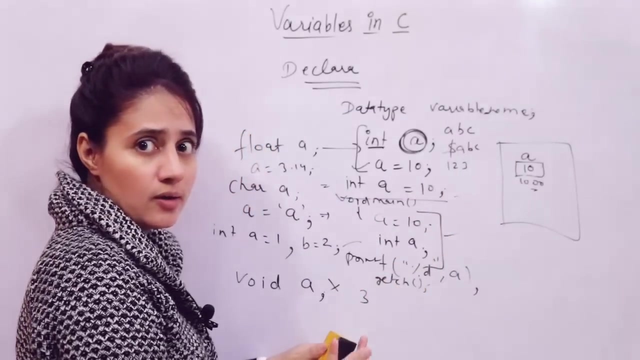 Now, while constructing the name of a variable, what you need to take care, What are some rules. See, suppose here I write like ABC, is it valid If I write $ABC? is it valid If I write 123, is it valid? 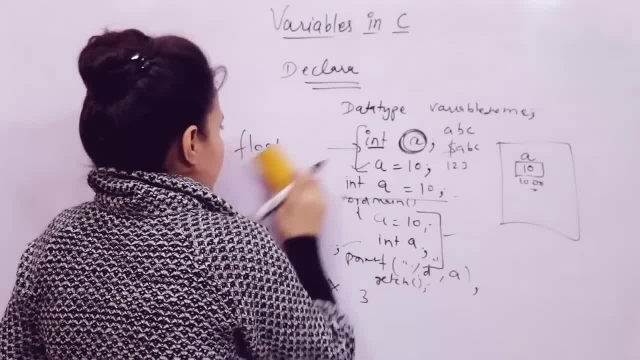 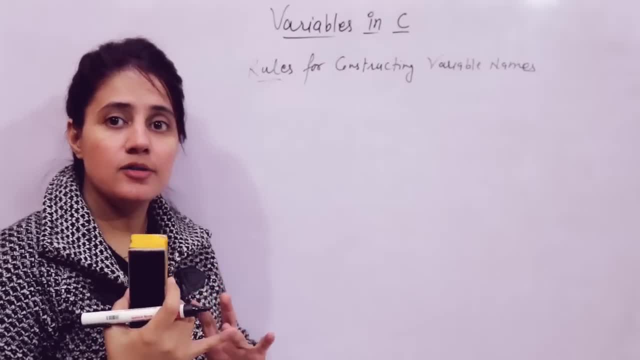 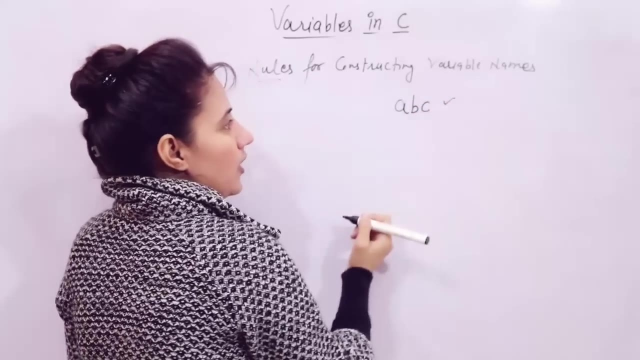 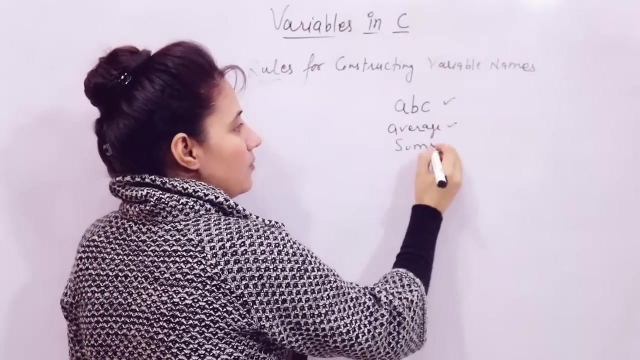 Let us check these rules. So a variable name may consist letters, digits and underscore a special symbol. So if I write, like here, ABC, yeah, this is valid. If I write here average, this is valid. If I write sum, this is valid. If I write sum12, this is also valid. 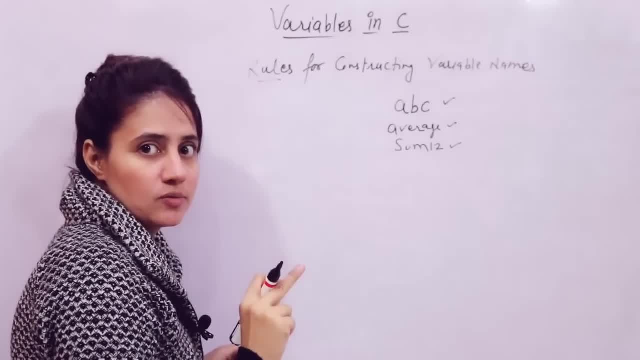 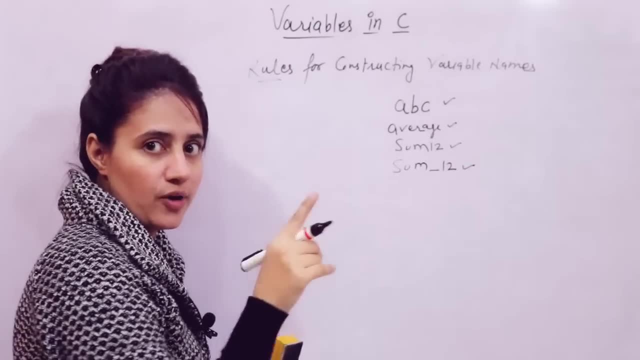 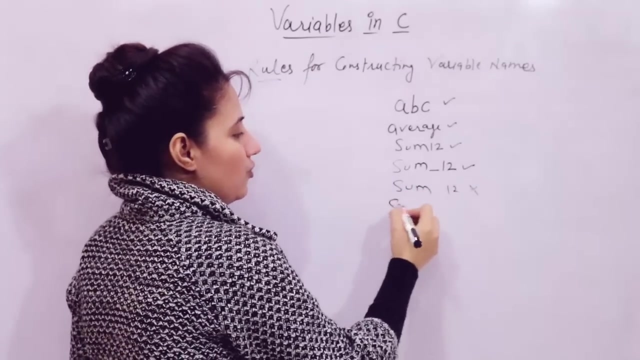 You can also write down numbers and letters And if I write down like sum underscore 12, this is also fine. valid underscore is allowed. But if you write sum space 12, this is invalid. If you write sum dollar 12, this is invalid. 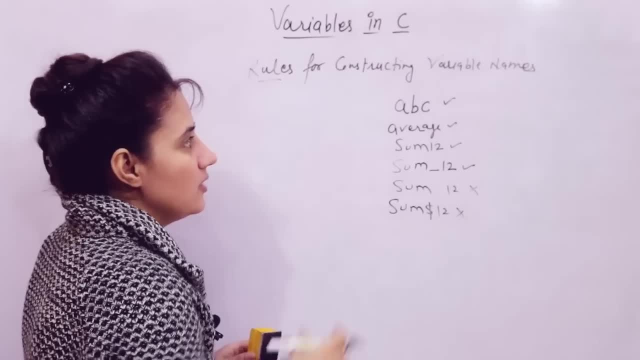 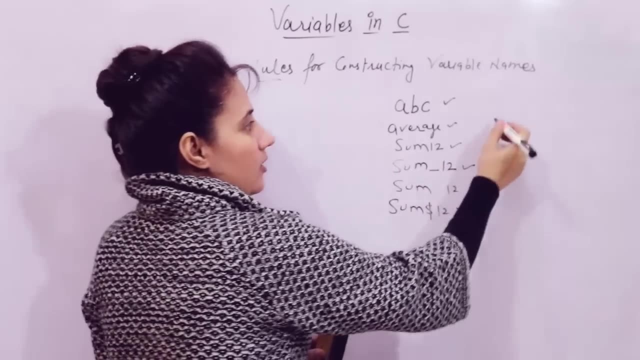 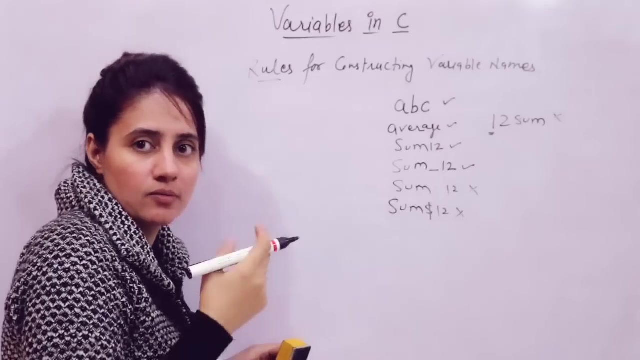 You cannot use any special symbol here. And second is: variable name also would be started from a letter. If I write like 1,, 2, sum, this is invalid. You cannot start it with a number. Yeah, Somewhere in some compiler it is valid that you can start it with underscore. 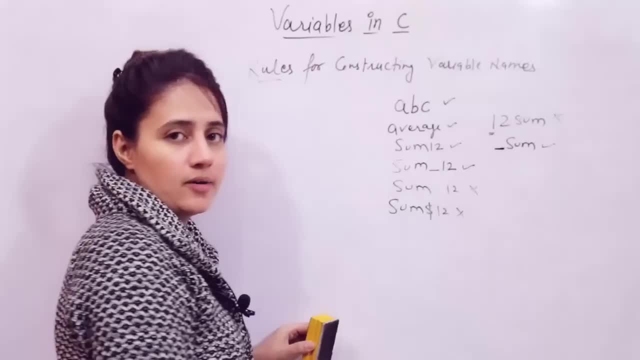 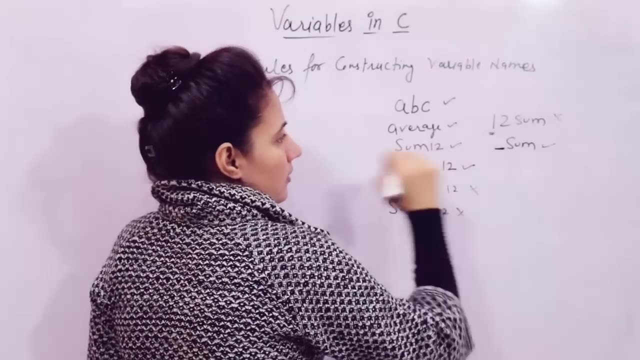 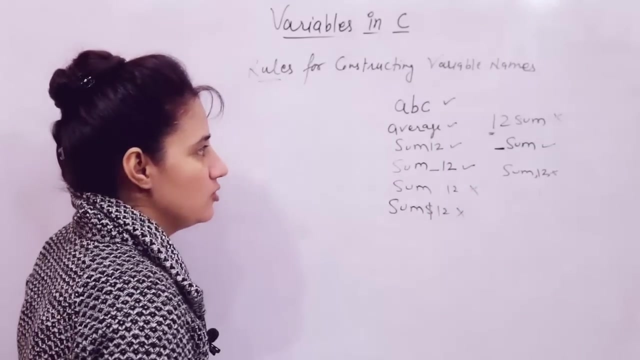 Underscore sum. this is valid right, Because some system permits underscore in the beginning right And you cannot write like sum, comma 12,. this is invalid. Comma is not allowed, space is not allowed. any special symbol is not allowed. underscore is allowed only. 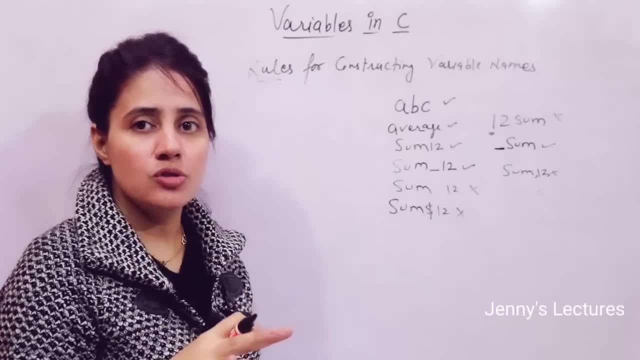 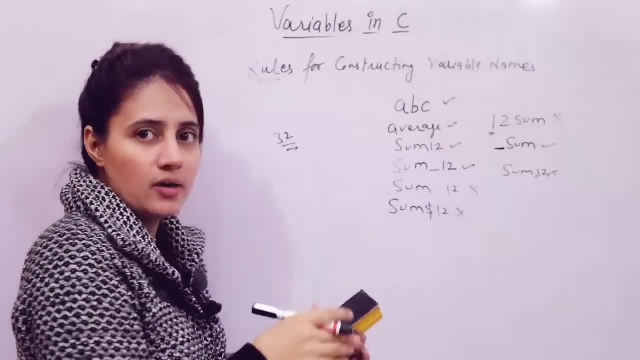 Next is: keyword cannot be used as a variable. Now, keywords are some reserved words in C. C is having what? 32 keywords? right, These are some reserved words and having some predefined meaning, So you cannot use those keywords as a variable name. 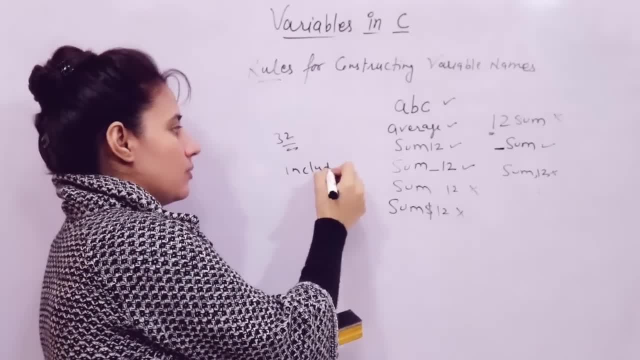 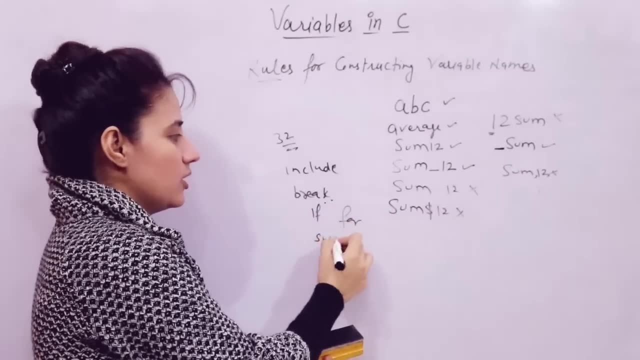 Like. you cannot use variable name include. You cannot use variable name break. This is a keyword. If is a keyword for, is a keyword. switch is a keyword. These are keywords that we will discuss in next video. What are the keywords? list of keywords: right. 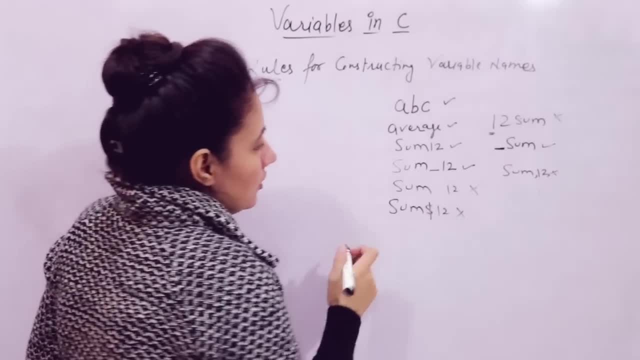 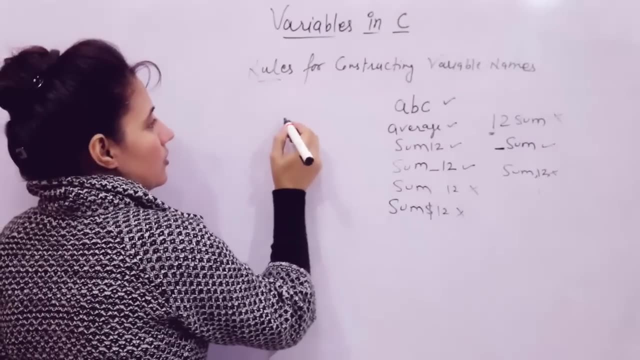 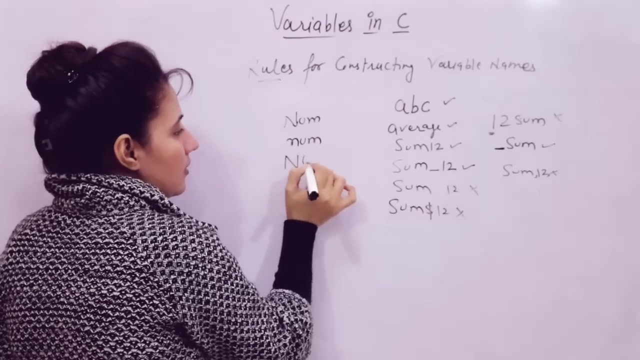 So next, keyword Keywords cannot be used as a variable name. Next is what Uppercase and lowercase letters are different, Like if I write here, suppose, num, and if I write num and if I write num. these three are different variables name.